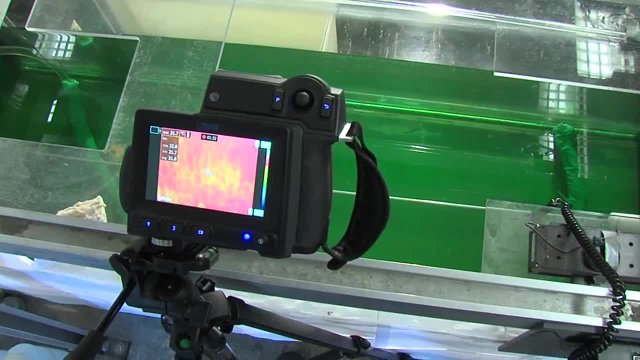 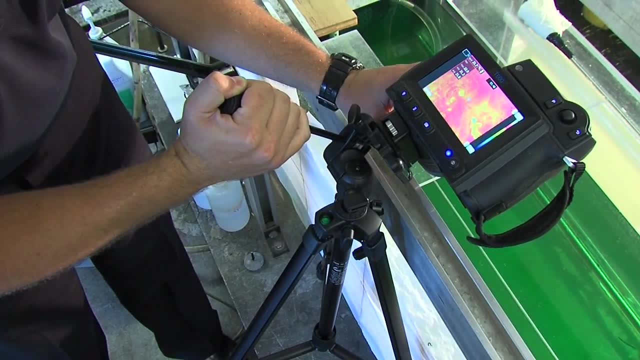 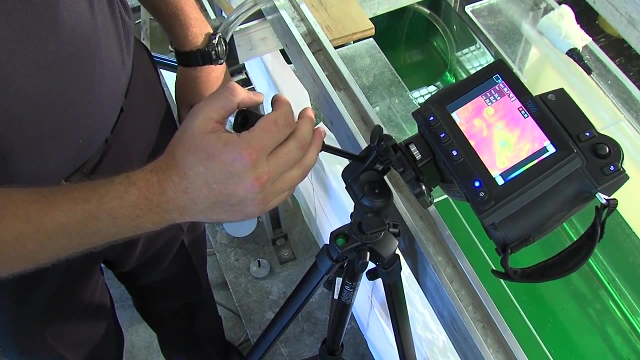 goes along this guide rod, it moves the water and causes internal waves which sometimes reach the surface, And you can see that with reflections in the infrared spectrum, Thermal spectrum. I need to know the temperature of the water at different levels, which is 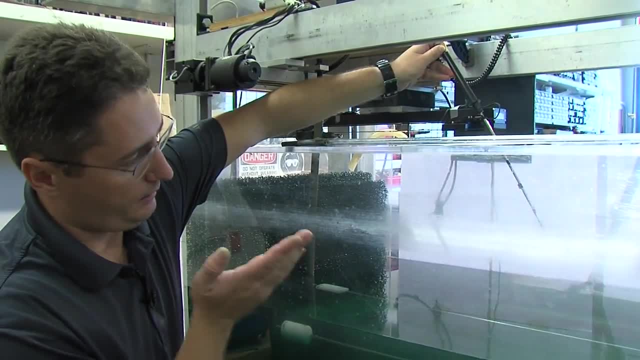 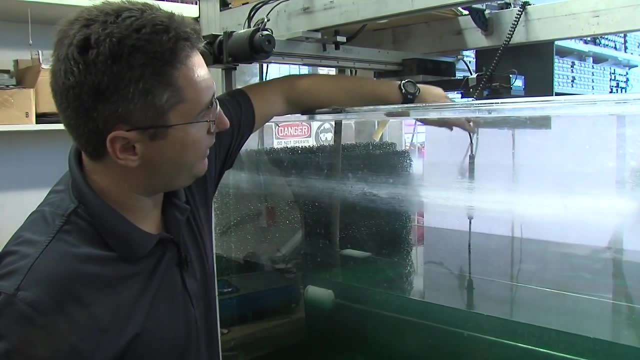 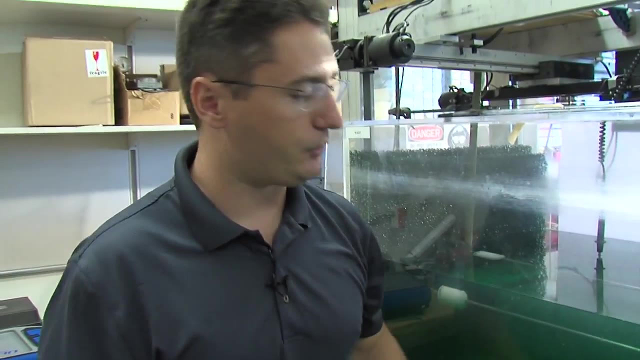 what I use this temperature probe for. I've got measurements marked every five centimeters, with the temperature being taken at the very tip, So I can suspend this at different levels within the tank, take a measurement and raise it up and create a temperature profile. The 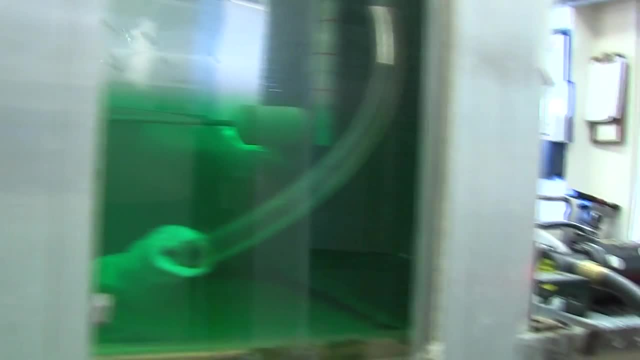 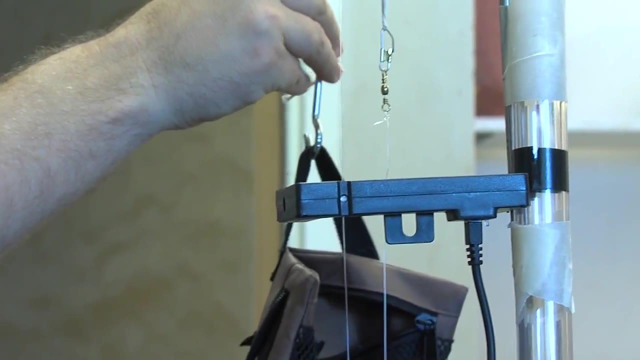 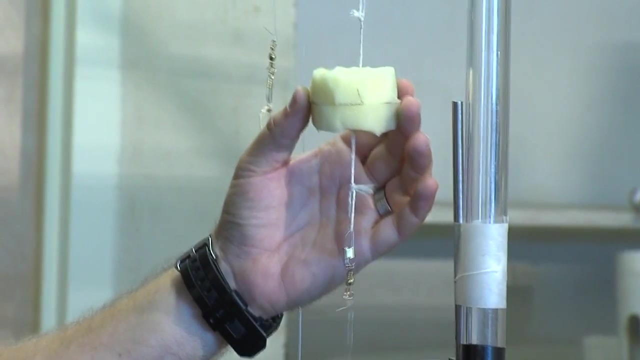 higher the velocity, the larger the wake. To control the velocity I've rigged up a tow line. I hang different amounts of weight from this hook and have it pull down. Heavier weight, faster speeds. To accurately measure the speed of the shuttle I've attached a little foam ball to the line that passes through. 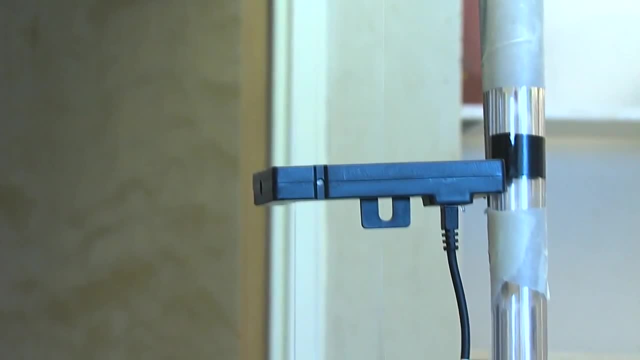 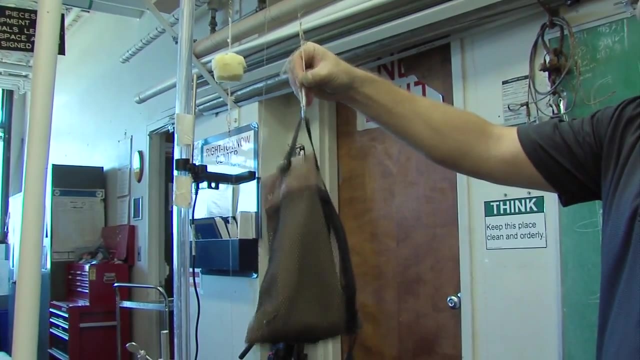 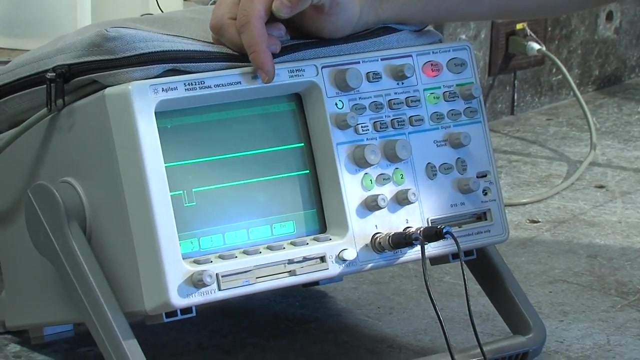 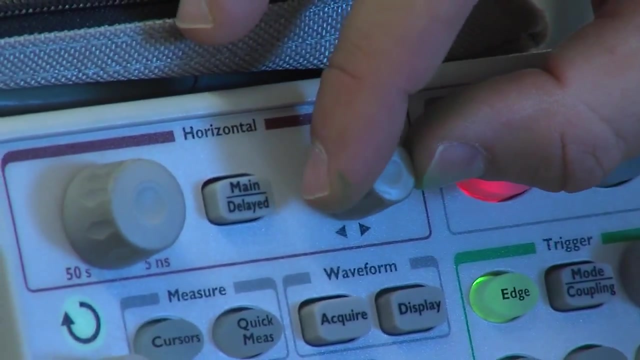 these photogates, which are light gates, So there's a laser passing between each arm of the photogates that, when broken, It starts the timer and stops the timer respectively. That time readout is seen on this oscilloscope by the drops in the two photogates and the signal. So I can see how much time had elapsed. 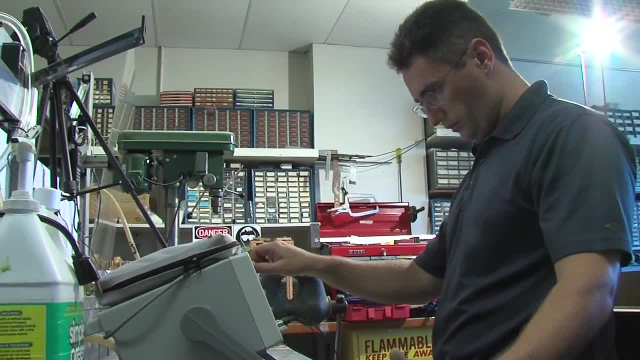 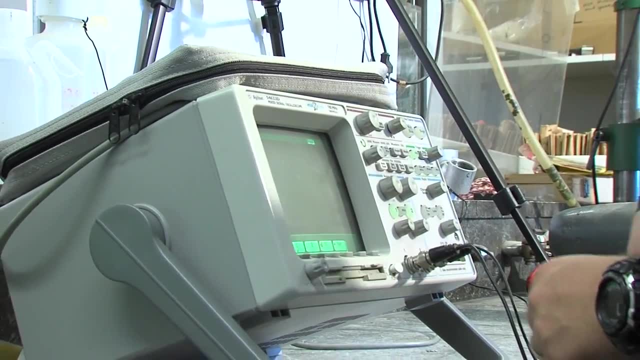 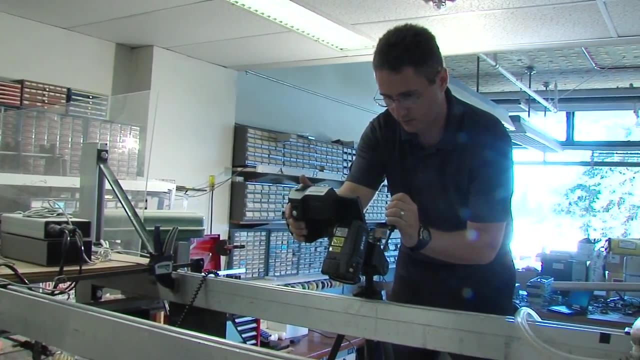 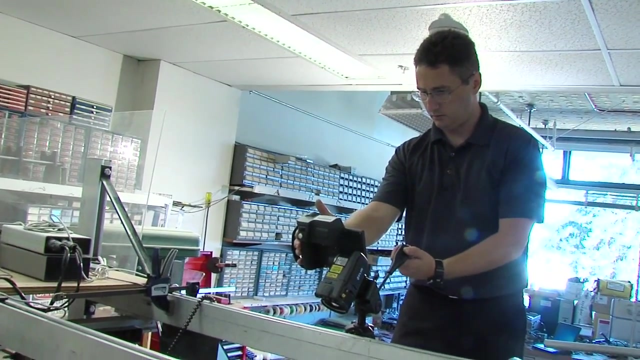 Since I know the distance between the two photogates, I can measure the time and then calculate the distance traveled over time, which is velocity. So, as I mentioned before, I am looking at the surface of the water using an infrared camera which detects heat. By looking from a top-down view, I'm able to see when the 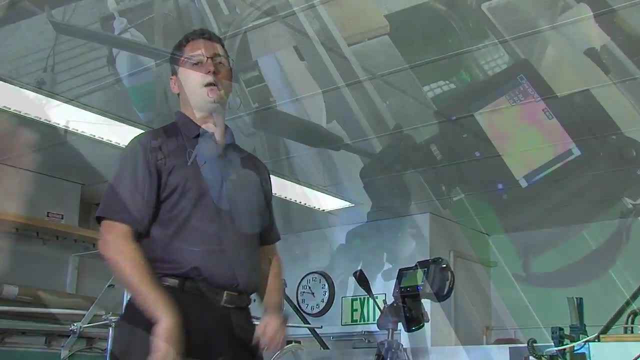 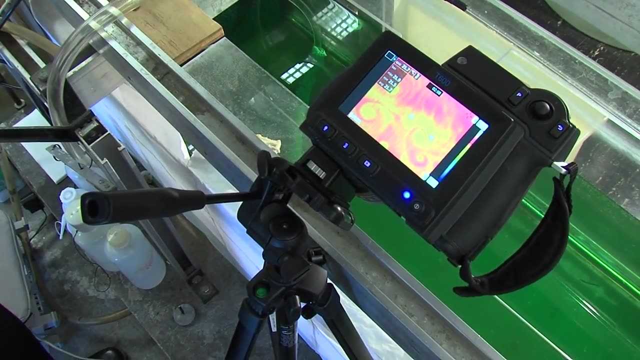 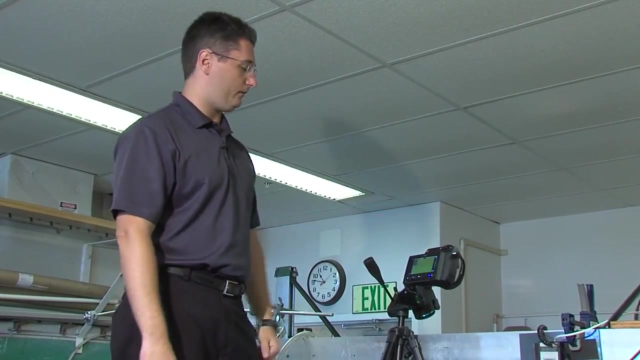 cold wake breaks the surface of the water And at that point I can see a thermal signature on the IR camera, where it's a little blue plume amongst the orange. I also have an actual temperature readout, of course, for the more precise measurements.